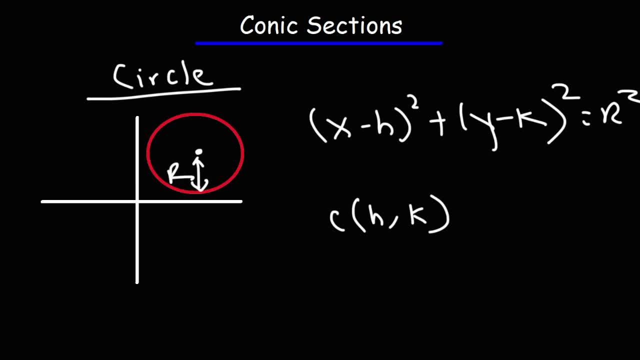 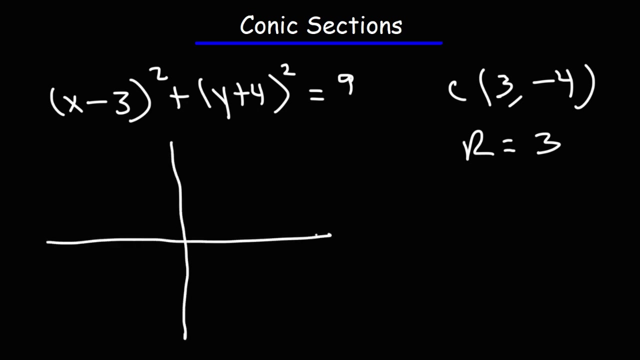 Now because graphing circles is very simple, let's do an example on this one. So let's say we have the equation x minus 3 squared plus y plus 4 squared. Let's say that's equal to 9. So h, to find it, simply change negative 3 to positive 3. To calculate k, change positive 4 to negative 4. So that's the center. It's 3 comma negative 3. four. The radius is the square root of that number. If r squared is nine, r is going to be the square root of nine or three. Now once you know the center and the radius, you can plot the circle. So let's begin by plotting the center. We need to travel three units to the right and then we need to go down four units. So it's here. Now the radius is three. To get the end point of the circle, we need to go up three units, three units to the left, then we need to go down three units from the center, and then we need to travel three units to the right. So those are the end points of the circle and then we simply need to connect them through a circle. Now my graph is not perfect but those are the basic steps that you would take in order to plot a circle. Plotting an ellipse is very similar to this. 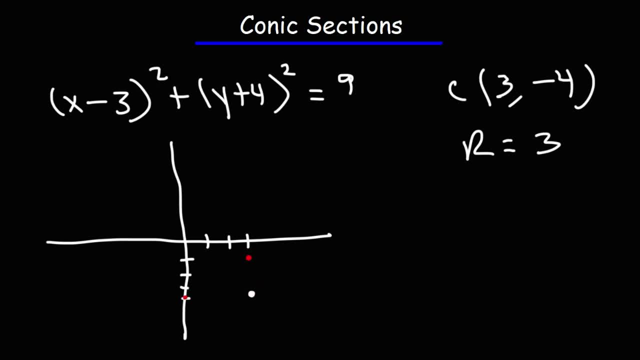 circle. we need to go up three units- three units to the left- then we need to go down three units from the center, and then we need to travel three units to the right. So those are the end points of the circle, and then we simply need to connect them through a circle. Now my graph is not perfect, but 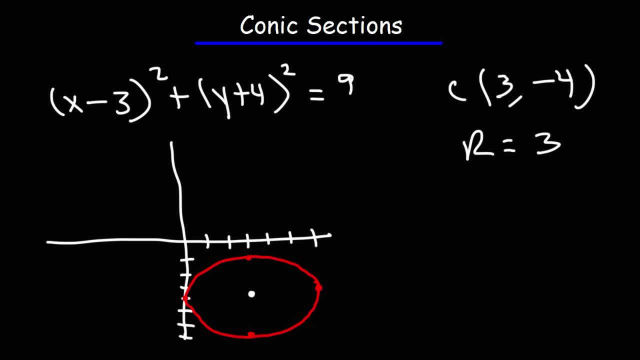 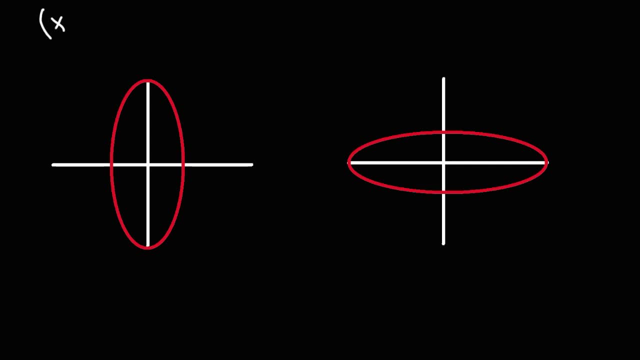 those are the basic steps that you would take in order to plot a circle. Plotting an ellipse is very similar to this. Now let's talk about ellipses. For the one on the left, the formula that corresponds to it is x minus. 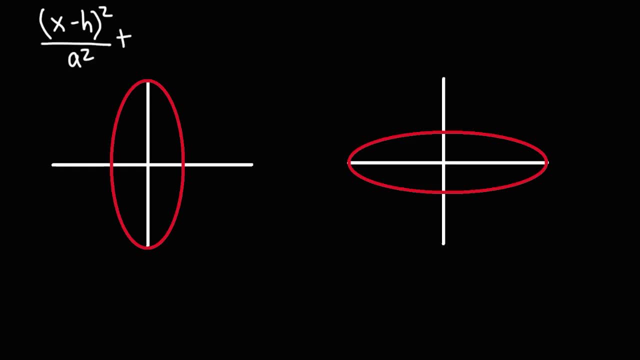 h squared over a squared plus y minus k squared over b squared, is equal to one. For the one on the right, it's x minus a squared over b squared, as opposed to a squared. So, as you can see, a and b have been reversed for these two types of ellipses. 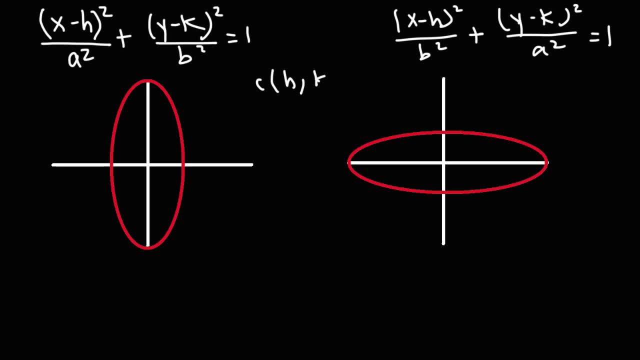 Now the center for both of them is still h comma k, very similar to the center of a circle. But the difference between an ellipse is it's an uneven circle. Now a is always bigger than b. That's how you can tell the two equations apart. 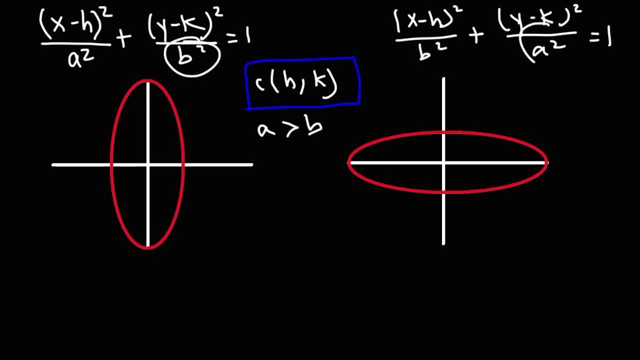 So if this value is larger, that's going to be your a squared. If the number under x minus h, squared, it is larger, that's your a squared. a is always bigger than b for ellipses. Now, a is the distance between the center and the major vertices. So these are the major vertices highlighted in white. 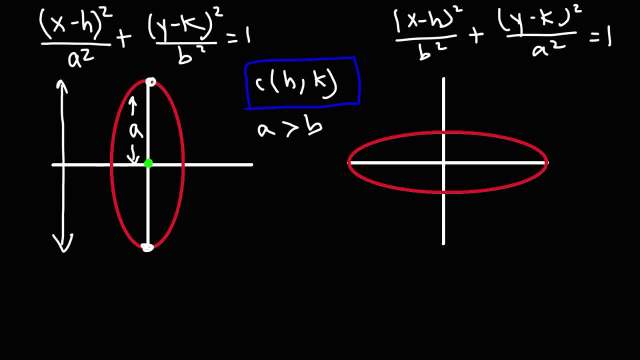 And this here is the axis. I mean it's the left of the major axis. The major axis is always equal to 2a. b is the distance between the center and the minor vertices, and the minor vertices are highlighted in blue here. The left of the minor axis is 2b. 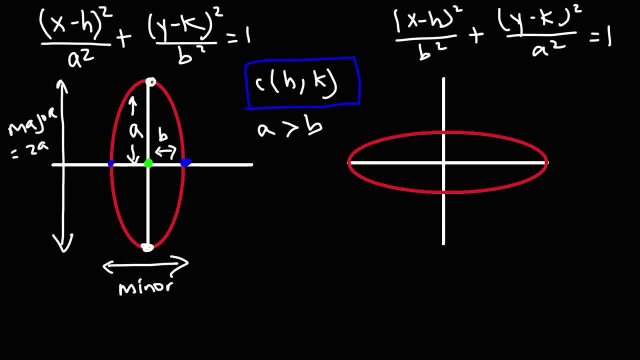 Now for the other one. the major axis is horizontal. Here the major axis is vertical on the left, but on the right the major axis is horizontal and it's always going to be equal to 2a. So, once again, a is the distance between the center and the major vertices. 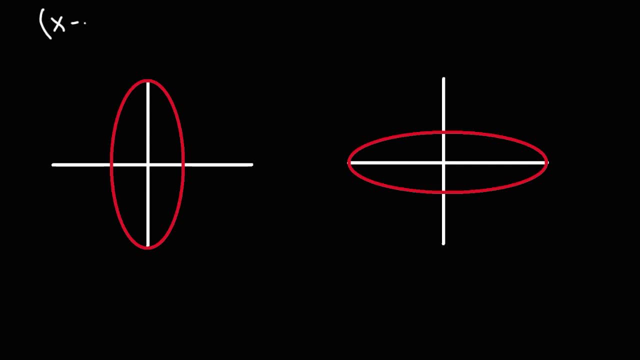 Now let's talk about ellipses. For the one on the left, the formula that corresponds to it is x minus h squared over a squared plus y minus k squared over b squared is equal to one. For the one on the right, it's x minus a squared over b squared as opposed to a squared. So as you can see, a and b have been reversed for these two types of ellipses. Now the center for both of them is still h comma k, very similar to the center of a circle. But the difference between an ellipse is it's an uneven circle. Now a is always bigger than b. That's how you can tell the two equations apart. So if this value is larger, that's going to be your a squared. If the number under x minus h squared is larger, that's your a squared. a is always bigger than b for ellipses. Now a is the distance between the center and the major vertices. So these are the major vertices highlighted in white. And this here is the axis, I mean it's the left of the major axis. 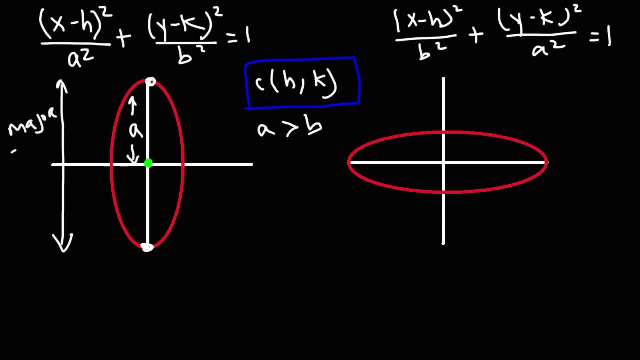 the major axis is always equal to 2a b is the distance between a center and the minor vertices and the minor vertices are highlighted in blue here the left of the minor axis is 2b now for the other one the major axis is horizontal here the major axis is vertical on the left 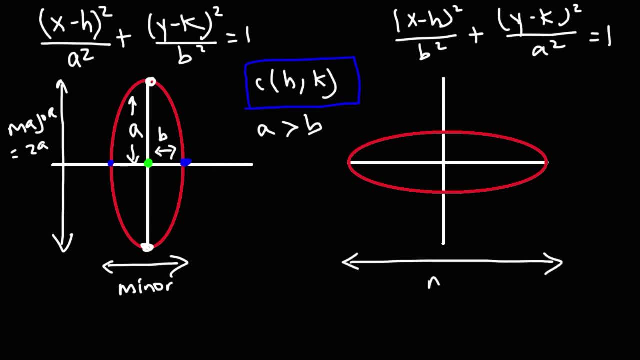 but on the right the major axis is horizontal and it's always going to be equal to 2a so once again a is the distance between a center and the major vertices so a is always the long part in the ellipse and the major vertices are highlighted here 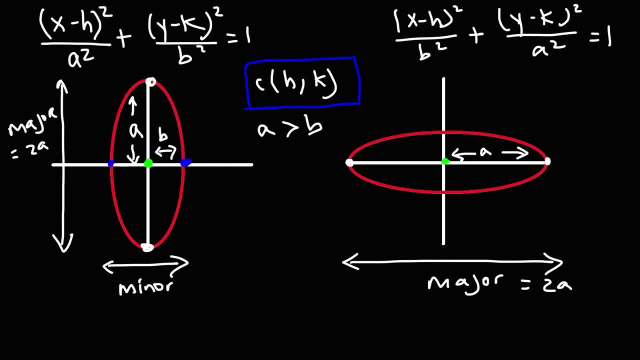 are now along the x-axis or parallel to it the minor vertices are along the y-axis if the center is centered at the origin so this is going to be B so it's important to calculate a and B when graphing ellipses because they can help you to find the vertices and thus plot the ellipse now 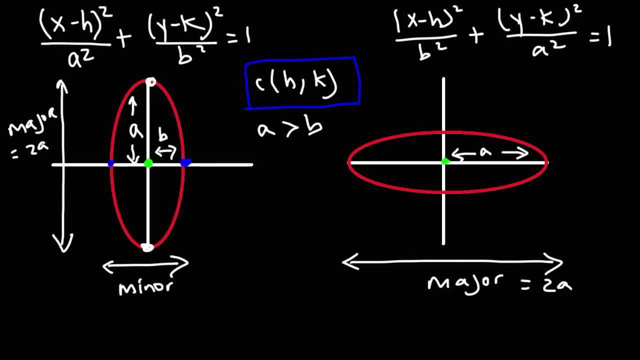 So a is always the long part in the ellipse and the major vertices are now along the x-axis or parallel to it. The minor vertices are along the y-axis if the center is centered at the origin. So this is going to be b. 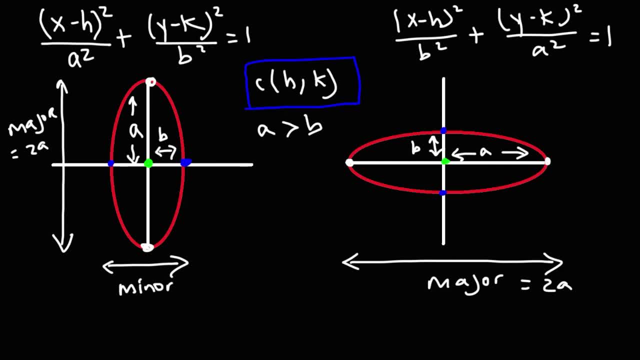 So it's important to calculate a and b when graphing ellipses, because they can help you define the vertices and thus plot the ellipse. Now, another thing we need to take into account is the value of c. c allows us to determine the foci. The foci is always along the major axis. 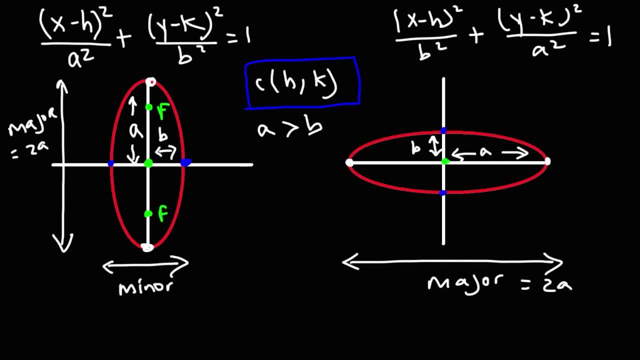 So let's put f for that. The distance between the center and the focus, or any one of the focus, is going to be c. So for the ellipse on the right the major axis is horizontal, So the foci will be along the major axis and it's going to be c units from the center. 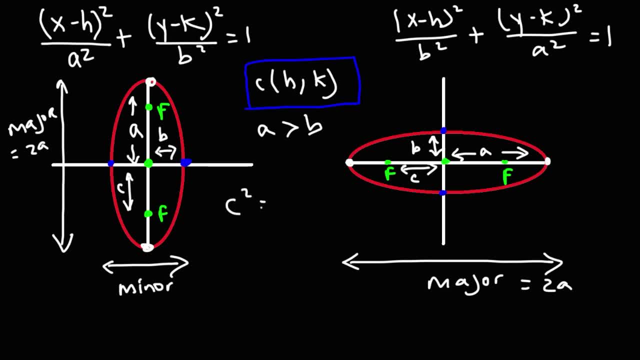 So to calculate c you need to use this formula: It's a squared minus b squared. It's not the Pythagorean theorem, a squared plus b squared, but a squared minus b squared. so remember, a is bigger than b and also a is bigger than c. 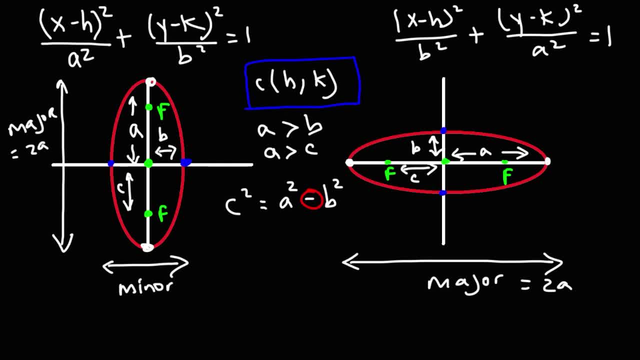 if you get a c value that's greater than a, you know you made a mistake. c has to be less than a. now, in order to determine the coordinates of the foci, here's what we need to do, or here's what can help you to get it, for whenever the axis is the major axis is vertical, it's going to be h comma. 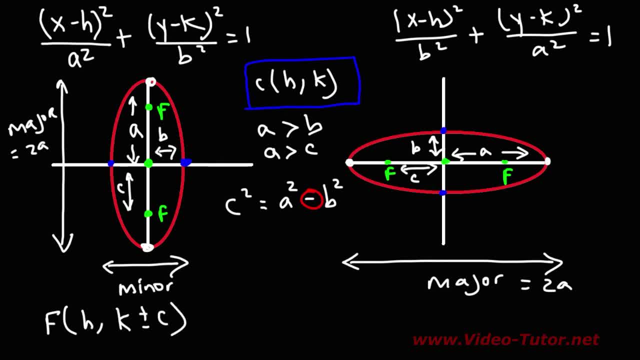 k plus or minus c. now let's understand why. remember, c is along the vertical axis, it's parallel to the y-axis. so thus you want to add and subtract c to the y-coordinate of the center of the ellipse. now for the ellipse on the right, the major axis is horizontal or parallel to the x-axis, so we're going to add: 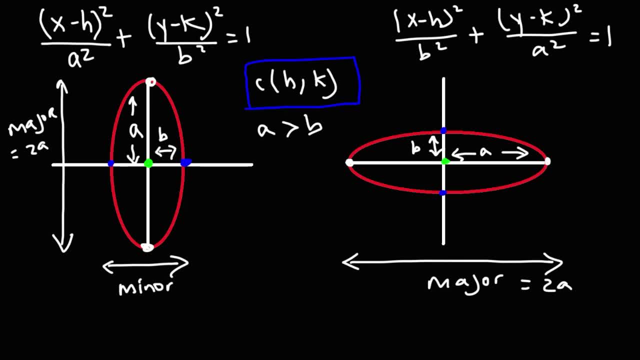 another thing we need to take into account is the value of C C allows us to determine the foci the foci is always along the major axis so let's put F for that the distance between the center and the focus or any one of the focus is going to be C so for the ellipse on the right the major axis is horizontal 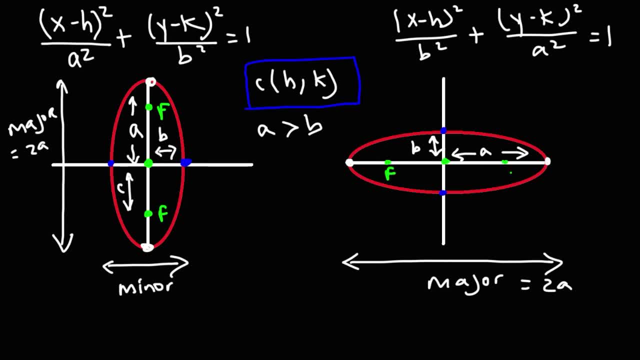 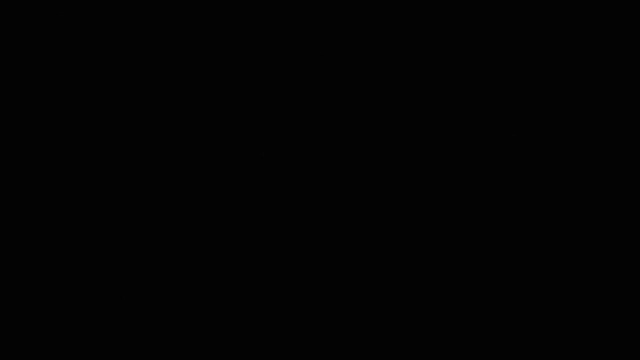 so the foci will be along the major axis and it's going to be C units from the center so to calculate C you need to use this formula it's a squared minus B squared it's not the Pythagorean theorem a squared plus B squared but a squared minus B squared so remember a is bigger than B and also a is bigger than C if you get a C though you that's greater than a you know you made a mistake C has to be less than A now in order to determine the coordinates of the foci here's what we need to do or his what can help you to get it for whenever the axis is the major axis is vertical it's going to be H comma K plus or minus C now let's understand why remember C is along the vertical axis it's parallel to the y axis so thus you want to add and subtract c to the y coordinate of the center of the ellipse now for the ellipse on the right the major axis is horizontal or parallel to the x-axis so we're going to add plus or minus c to the x-coordinate of the center so that's how you can determine the coordinates of the foci for these two different types of ellipse now let's talk about finding the area of an ellipse but first let's find the area of a circle so this is the center of the circle and this is the radius and this is also the radius the area of a circle is pi r squared you could think of it as pi times the first r 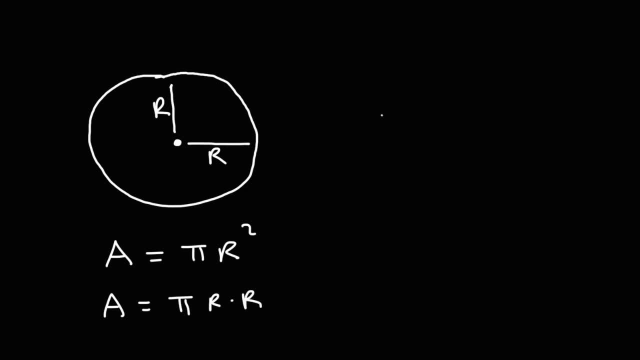 times the second r now let's compare this to an ellipse okay that's a terrible looking ellipse let's do that again 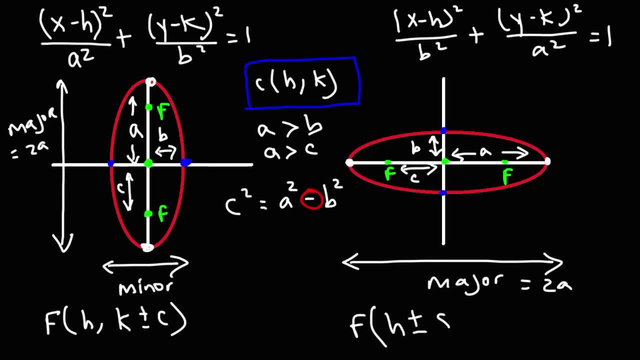 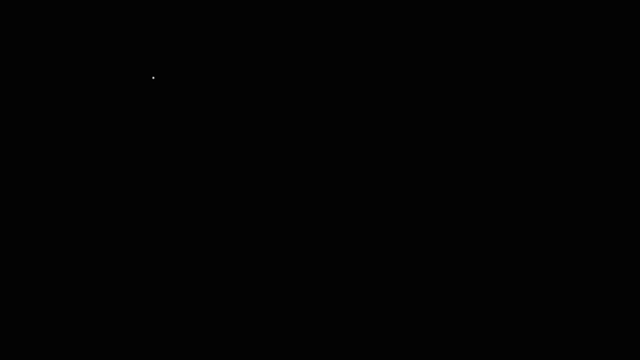 plus or minus c to the x-coordinate of the center. so that's how you can determine the coordinates of the foci for these two different types of ellipse. now let's talk about finding the area of an ellipse, but first let's find the area of a circle. so this is the area of an ellipse. 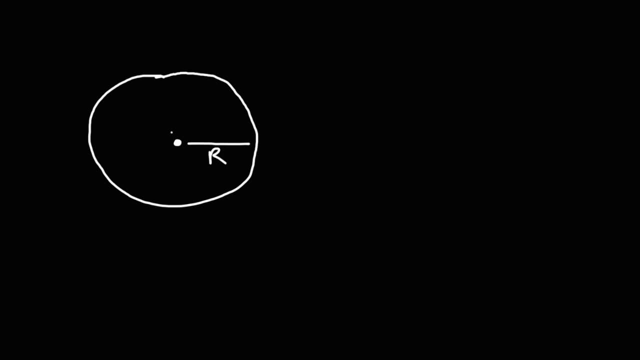 so this is the center of the circle and this is the radius, and this is also the radius. the area of a circle is pi r squared. you could think of it as pi times the first r times the second r. now let's compare this to an ellipse. okay, that's a terrible looking ellipse. let's do that again. 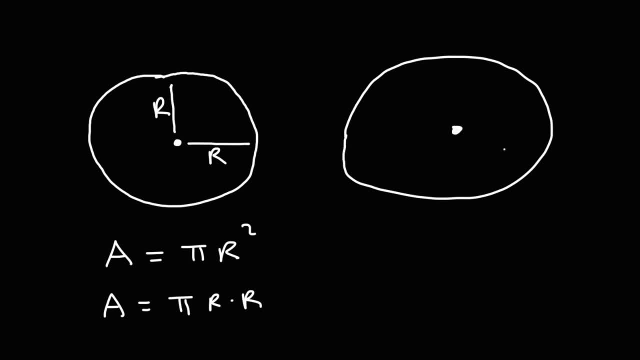 all right, we'll work with that. so let's say: this is the center, this is going to be a and this is going to be b. the major axis is horizontal, so the equation is going to be very similar to this one, but instead of pi times r times r. r is not the same here it's different. it's going to be pi times a times b. 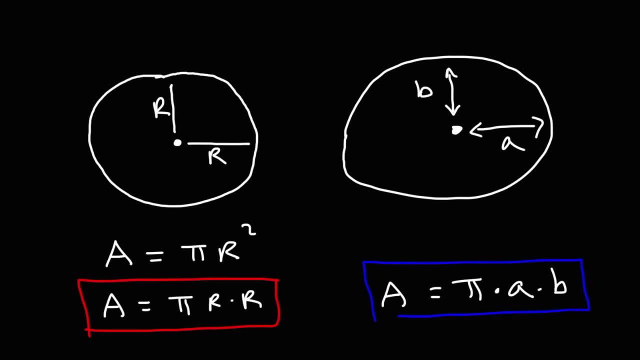 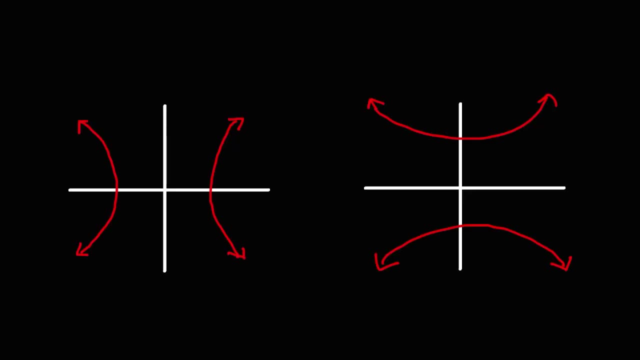 so that's how you could do this. let's see how you can determine. the area of an ellipse is very similar to the area of the circle, but because the circle is uneven, you know, it's not going to be r times r, it's going to be a times b. the next type of graph we need to talk about is the hyperbola. for the one on the left it corresponds to this formula: x minus h, squared over a squared, minus y minus k squared over b squared, is equal to 1. 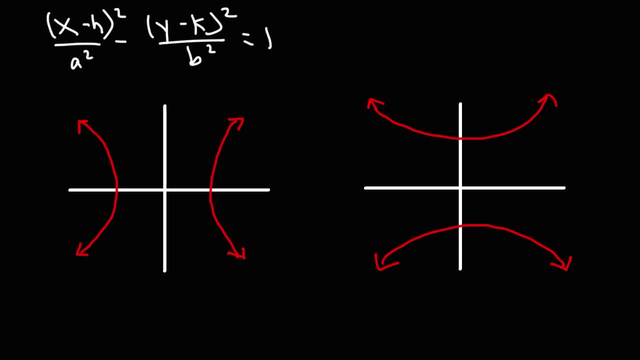 notice the difference between this and the ellipse. with the ellipse there's a plus sign, but with the hyperbola there's a minus sign. now for the hyperbola on the right. the equation is: y minus k squared over a, squared minus x minus h squared over b, squared is equal to 1. 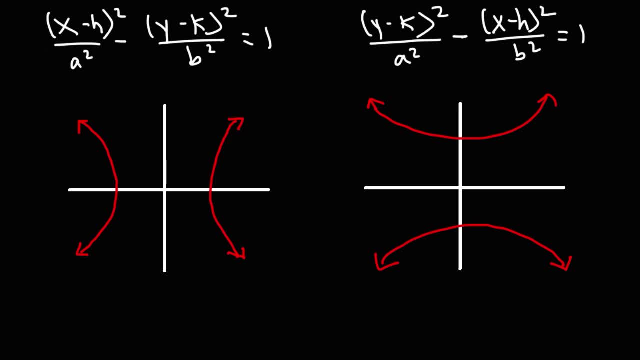 so if x squared is positive, it's going to open to the left and to the right. if y squared is positive, it's going to open up and down. so that's how you can determine the direction in which the hyperbola opens. a is the distance between the center. 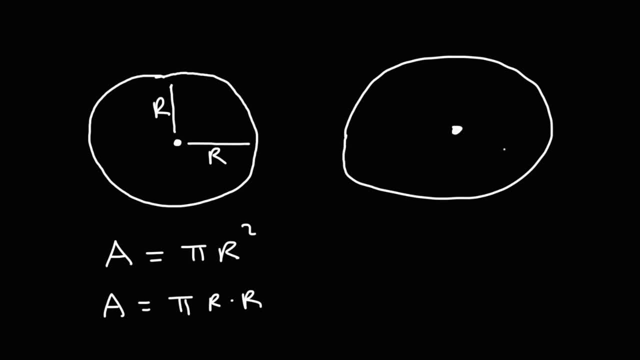 all right we'll work with that so let's say this is the center this is going to be a and this is going to be b the major axis is horizontal 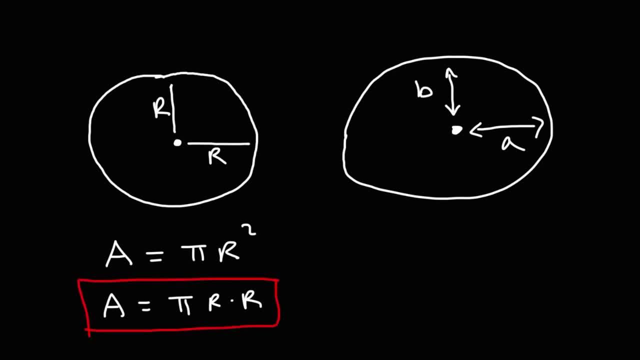 so the equation is going to be very similar to this one but instead of pi times r times r r is not the same here it's different it's going to be pi times a 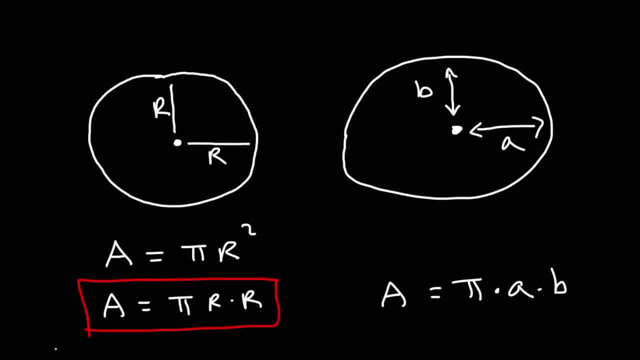 times b so that's how you could determine the area of an ellipse is very similar to the area of the circle but because the circle is uneven you know it's not going to be r times r it's going to be 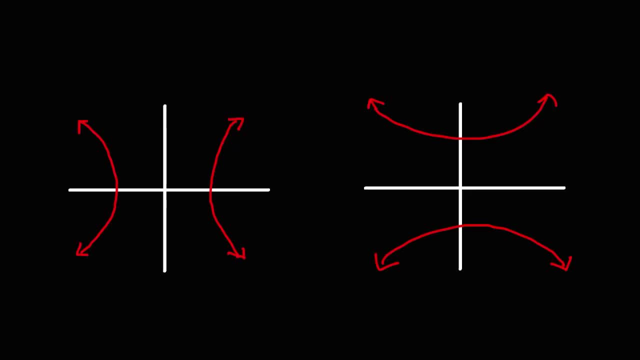 a times b the next type of graph we need to talk about is the hyperbola so we're going to talk about 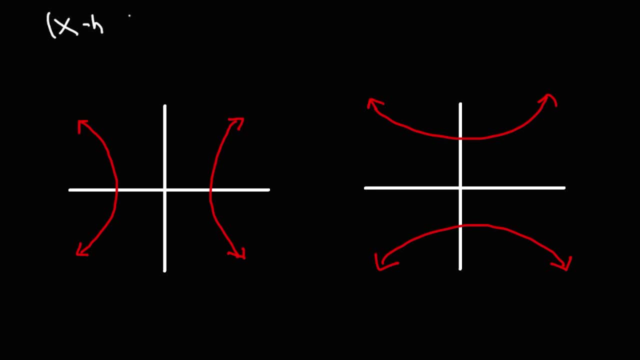 the operator Elitey in a little bit later but the formula for the und wardrobe is just basically the ampere square root of the variableի 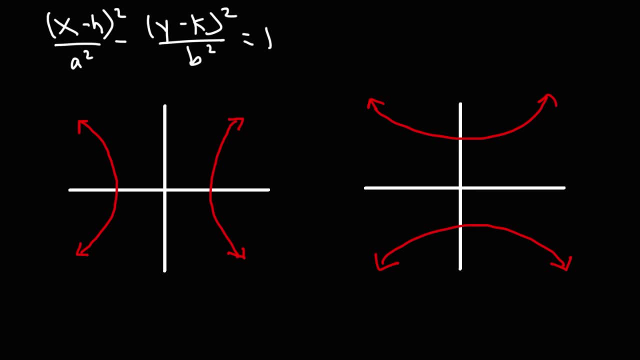 so here's what we need this formula means for the one on the left it corresponds to this formula x minus h squared over a squared minus 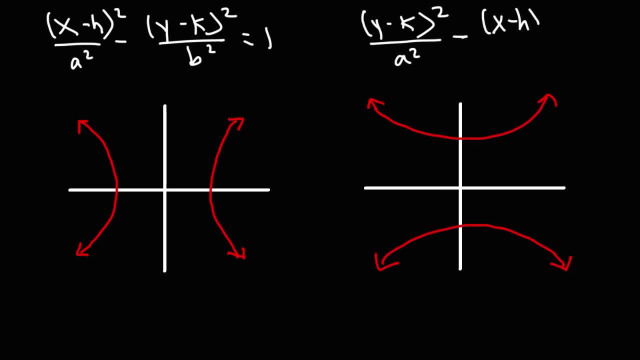 over a squared minus x minus a squared over b squared is equal to 1. 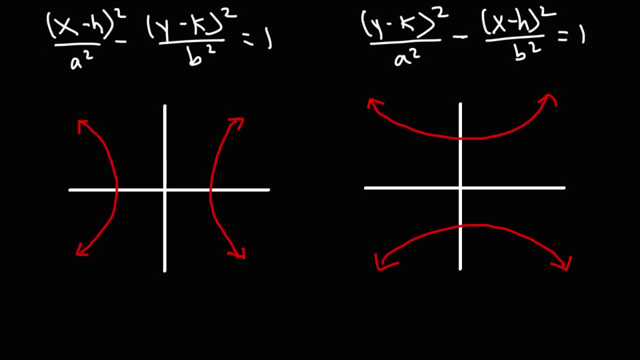 So if x squared is positive, it's going to open to the left and to the right. If y squared is positive, it's going to open up and down. 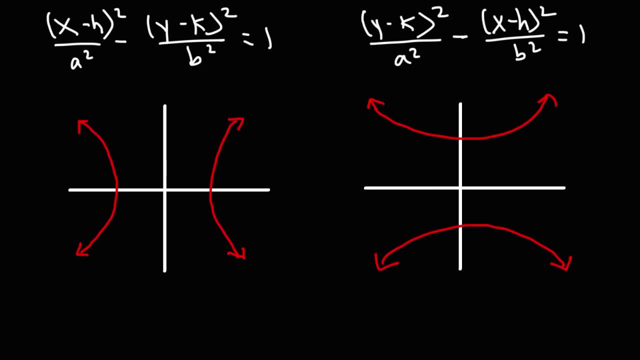 Next, a is the distance between the center and the vertex. Now there's two vertex, so it's the distance between the center and the vertices. 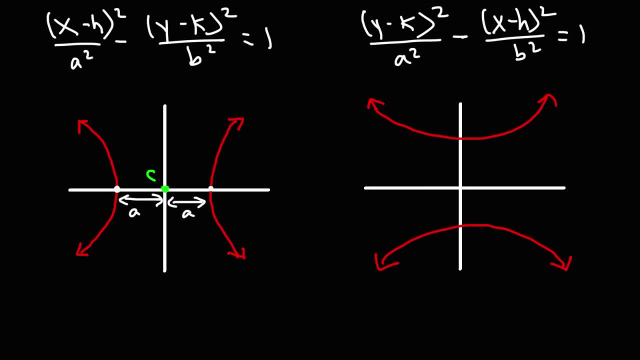 So here are the vertices of the hyperbola. To find the coordinates of the vertices, you can use this. 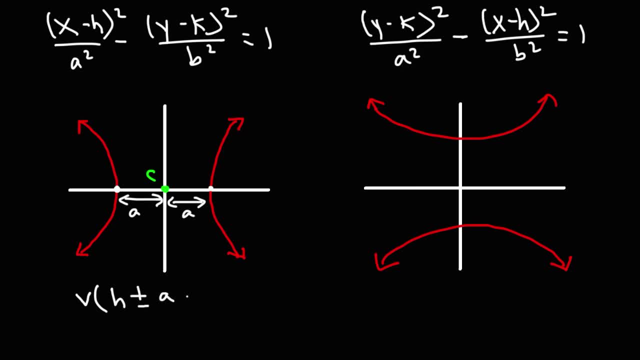 It's going to be h plus or minus a comma k. Because a is the distance between the center and the vertex. 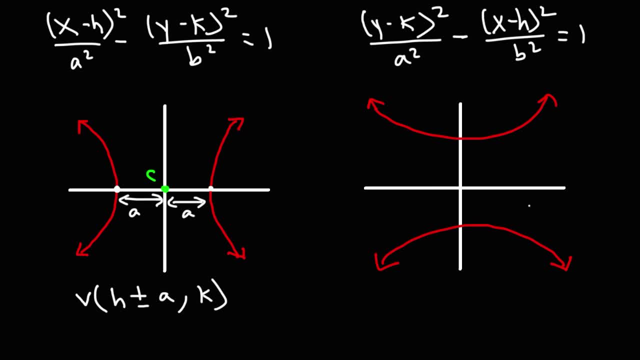 So a is horizontal for the hyperbola on the left. On the right, a is vertical. a is the distance between the center and the vertices. 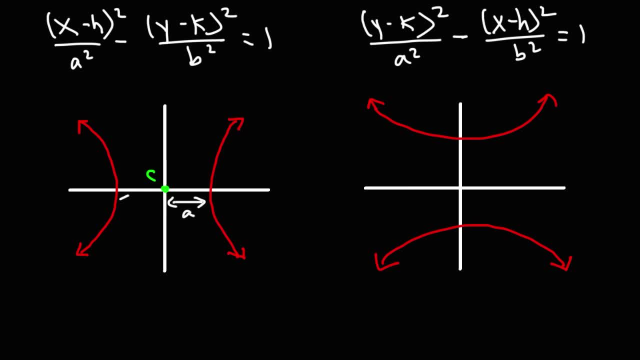 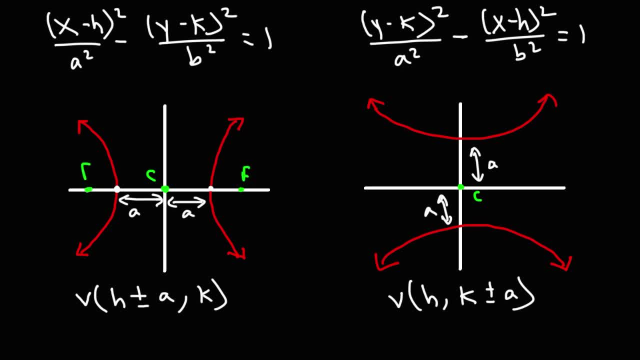 The foci. you can find them where the hyperbola opens up towards. It always opens towards the foci. And C, not the center, C, but the value C is the difference between the center and the foci. So to find the coordinates of the foci, it's going to be H plus or minus C, comma, K. 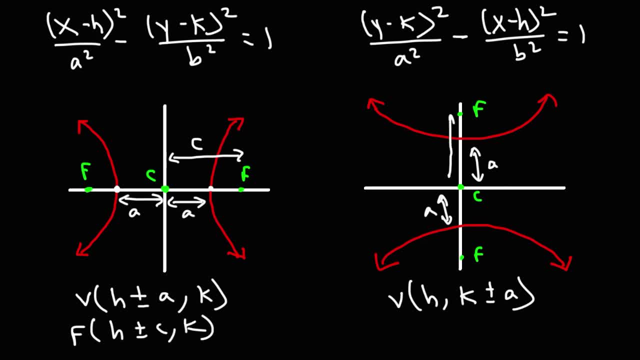 Now for the hyperbola on the right. C is vertical, So we're going to add and subtract C from K, And this should be an F, not a V. So that's how you can find the coordinates of the foci when dealing with a hyperbola. 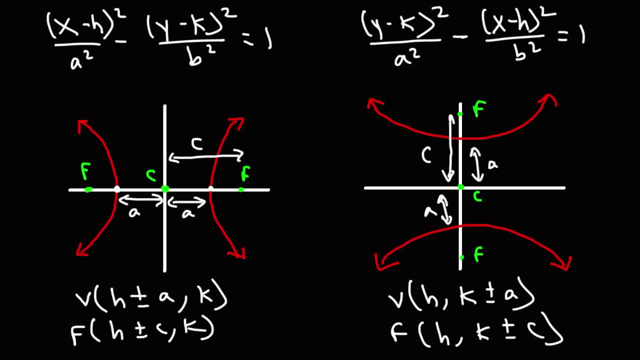 Now the last thing we need to talk about is finding the equation of the asymptotes. So let me clear away a few things. So, when plotting a hyperbola, you would find the center, travel A units to the right to get the vertex on the right, A units to the left, and then you would also travel B units up and down. 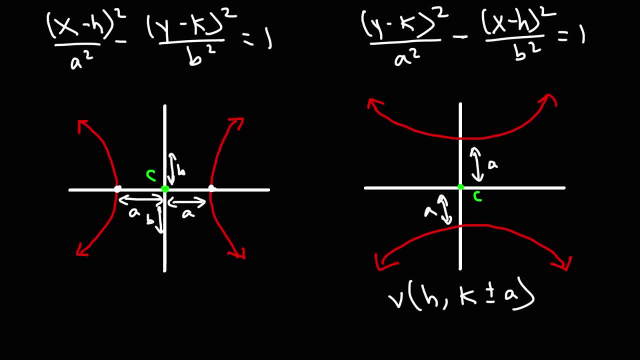 This is just a rough sketch, by the way. And then, once you have A and B, you can find the coordinates of the asymptotes. So, once you have A and B, what you want to do is you want to plot a rectangular dotted box. 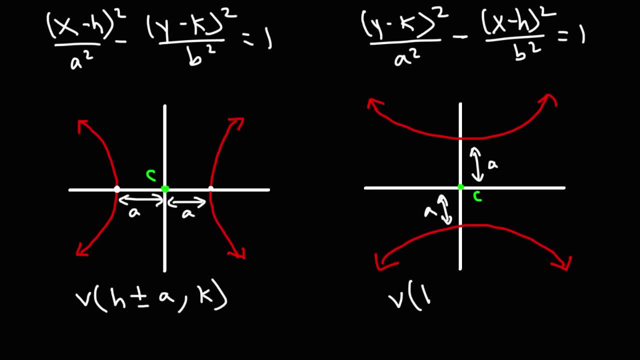 So in this case, the coordinates of the vertices will be h comma k plus or minus a. 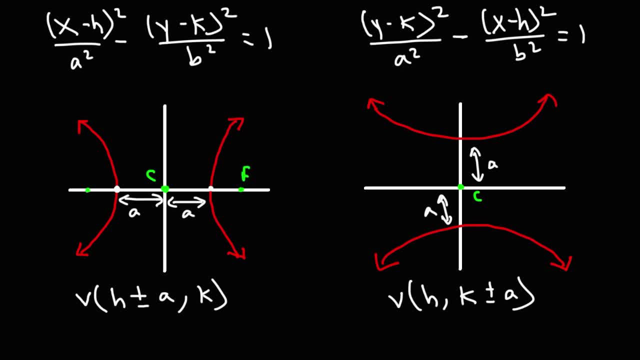 Now, the foci, you can find them where the hyperbola opens up towards. It always opens towards the foci. 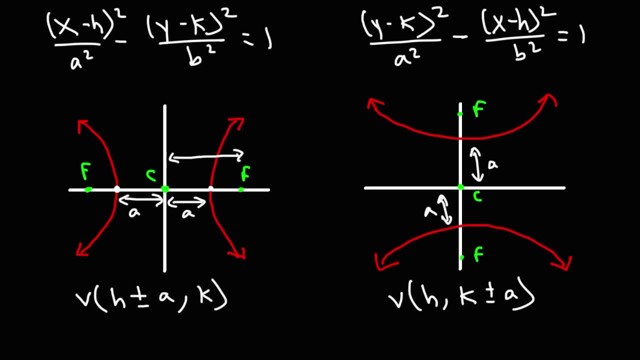 And c, not the center c, but the value c is the difference between the center and the foci. So to find the coordinates of the foci, it's going to be h plus or minus c comma k. 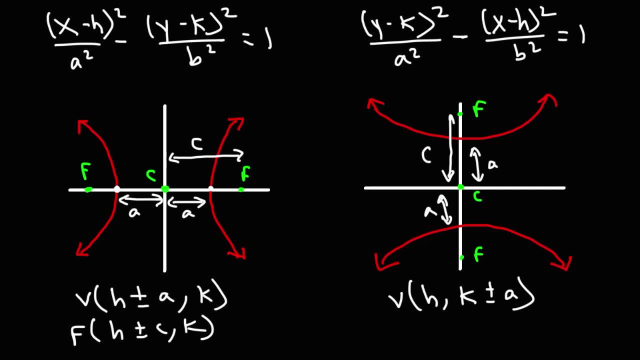 Now for that hyperbola on the right, c is vertical. 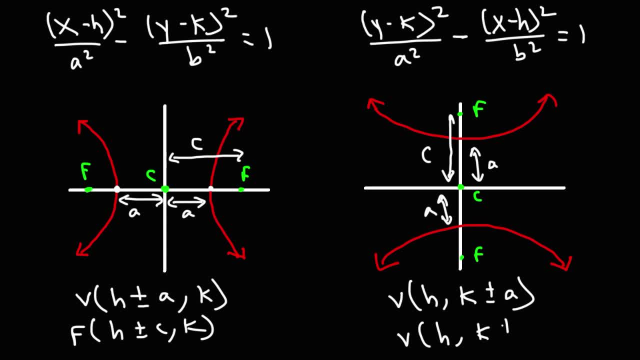 So we're going to add and subtract c from k. And this should be an f, not a v. So that's how you can find the coordinates of the foci when dealing with a hyperbola. 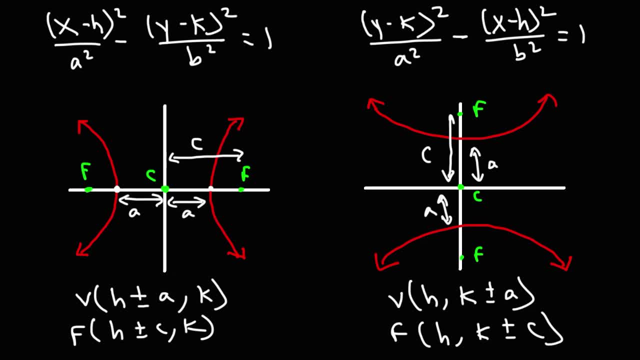 Now the last thing we need to talk about is finding the equation of the asymptotes. So let me clear away a few things. 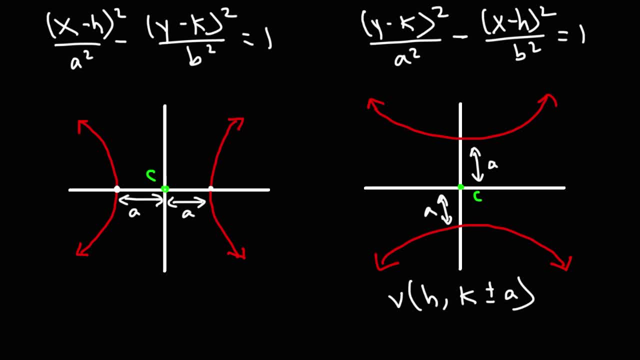 So when plotting a hyperbola, you would find the center, travel a units to the right to get the vertex on the right, a units to the left, and then you would also travel b units up and down. This is just a rough sketch, by the way. And then once you have a and b, what you want to do is you want to plot a rectangular dotted box. And then what you're supposed to do is you would plot the asymptotes, which goes from one diagonal of the box through the center to the other corner of the box. 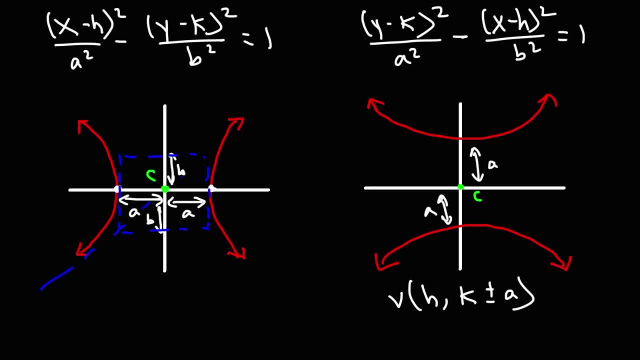 And then what you're supposed to do is you would plot the asymptotes which goes from one diagonal of the box through the center, to the other corner of the box. So you draw these diagonals that go from one corner of the box to the other corner through the center. 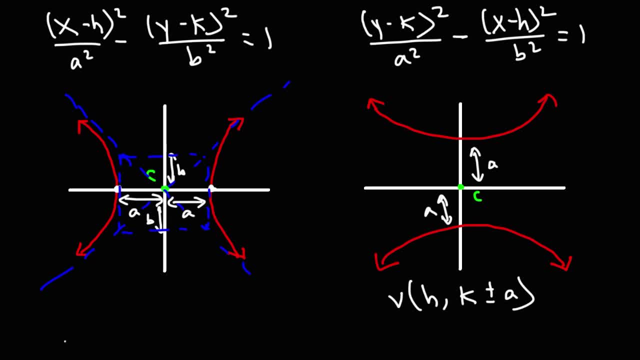 And then you would plot the asymptotes, And then you would plot the asymptotes And then to find the equation of those two asymptotes, it's going to be Y minus K. basically, what you see here equals now the slope Starting from the center. the slope is the rise over the run. 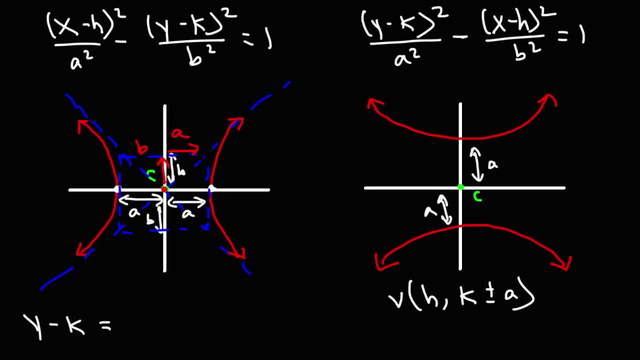 So we rose B units and travel or ran A units to the right. So the slope is going to be plus or minus B over A, and then what we see here: X minus H. Now the reason we have, The reason we have plus or minus, is the first diagonal has a positive slope. 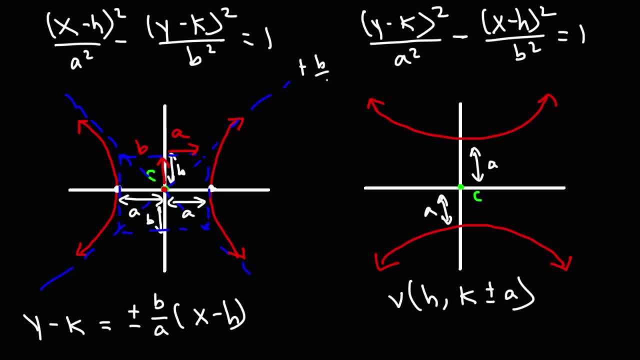 So that's going to be the equation that corresponds to positive B over A. The second diagonal has a negative slope, So that's the second equation that corresponds to negative B over A. That's what we have too, because there are two asymptotes, one with a positive slope and the other with a negative slope. 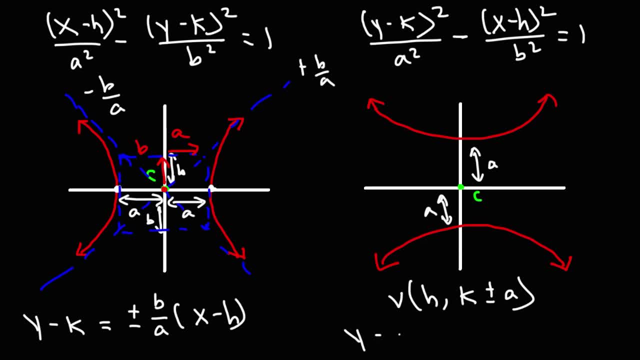 Now for the hyperbola on the right. the equation of the asymptotes will be Y minus K. So we rise. K equals plus or minus. Notice the slope is different This time. the rise is A, the run is going to be B. 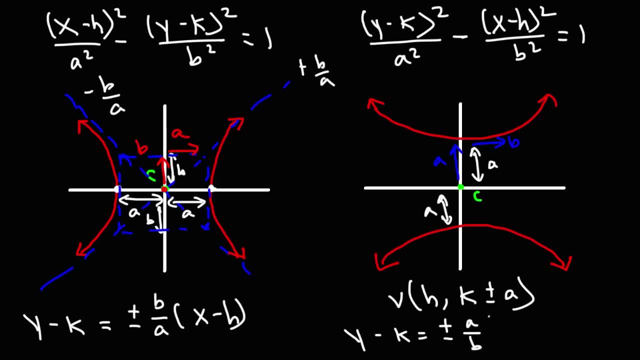 So instead of plus or minus B over A, it's now plus or minus A over B, and then X minus H. So that's the difference between the asymptotes of these two types of hyperbolas. The difference is in the slope. 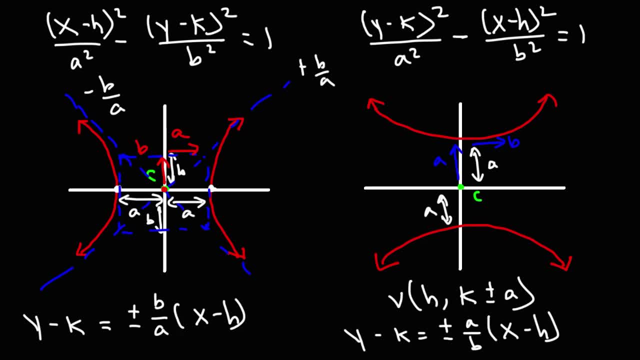 In one case it's B over A, in the other case it's A over B. If you ever forget, it's always going to be the rise over the run. Now we talked about finding the coordinates of the foci by calculating the value of C or using C to find it. 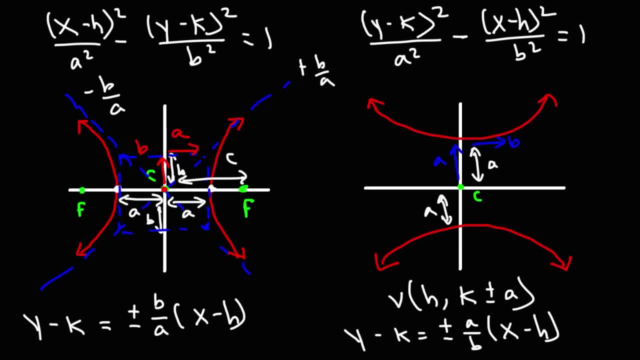 Now we need to talk about how to find C. With the ellipse, we said that A was larger than C. With the hyperbola, C is going to be larger than A, So C squared is going to be not A squared minus B squared, but A squared plus B squared. 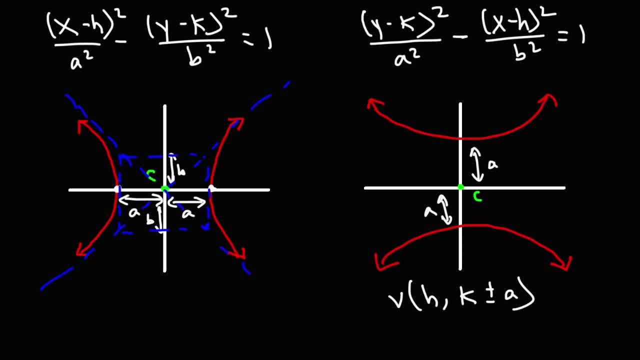 So you draw these diagonals that go from one corner of the box to the other corner to the center. And then to find the equation of those two asymptotes, it's going to be y minus k, basically what you see here, equals now the slope. Starting from the center, the slope is the rise over the run. So we rose b units and travel or ran a units to the right. So the slope is going to be plus or minus b over a, and then what we see here, x minus h. Now the reason we have plus or minus is the first diagonal has a positive slope. So that's going to be the equation that corresponds to positive b over a. The second diagonal has a negative slope. So that's the second equation that corresponds to negative b over a. 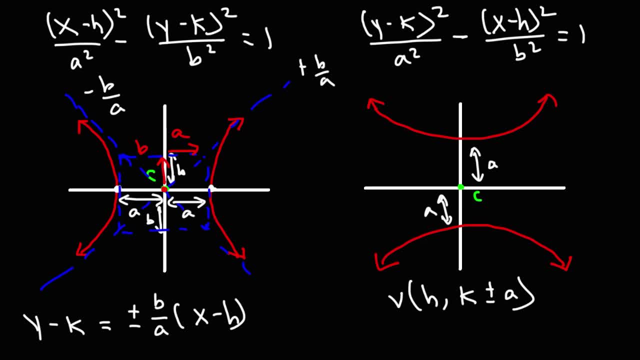 That's what we have too, because there are two asymptotes, one with a positive slope and the other with a negative slope. 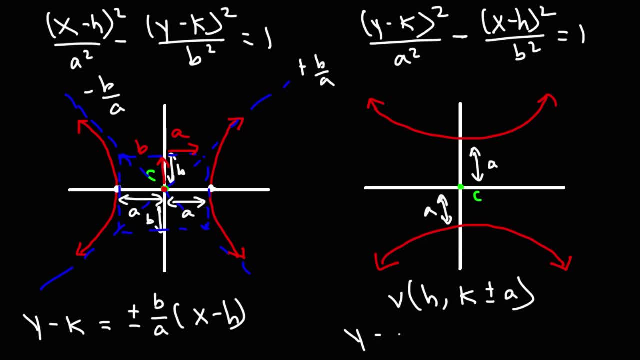 Now for the hyperbola on the right, the equation of the asymptotes will be y minus k equals plus or minus. Notice the slope is different. This time, the rise is a, the run is going to be b. So instead of plus or minus, we're going to have a negative slope. So instead of plus or minus, we're going to have a negative slope. So instead of plus or minus, we're going to have a negative slope. 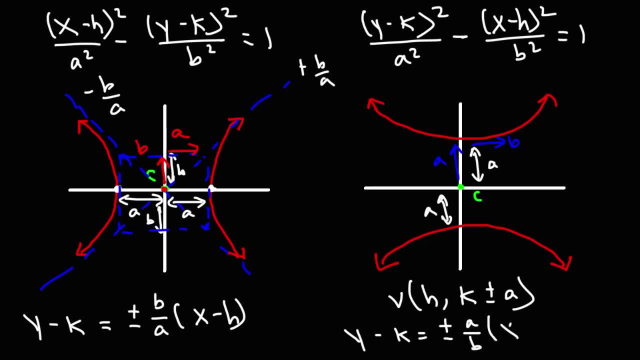 So instead of plus or minus b over a, it's now plus or minus a over b, and then x minus h. So that's the difference between the asymptotes of these two types of hyperbolas. 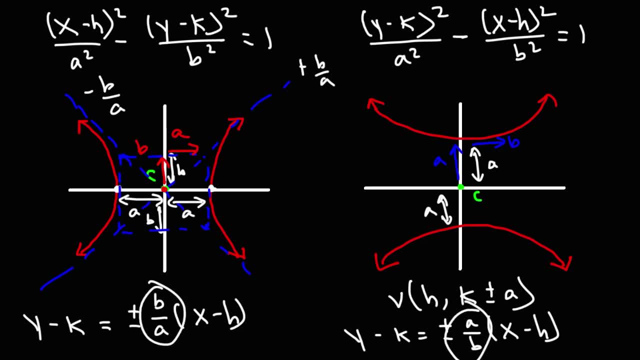 The difference is in the slope. In one case, it's b over a. In the other case, it's a over b. If you ever forget, it's always going to be the rise over the run. 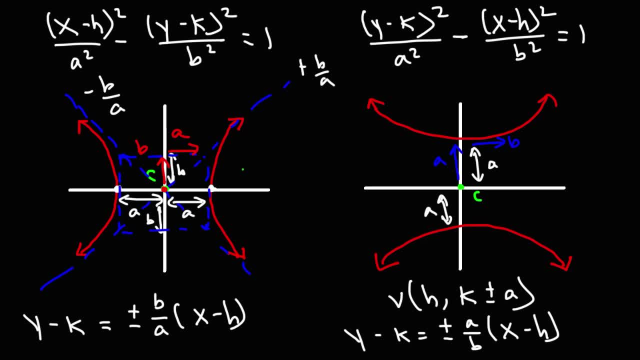 Now, we talked about finding the coordinates of the foci by calculating the value of c. Or, using c to find it. Now, we need to talk about how to find c. With the ellipse, we said that a was larger than c. With the hyperbola, c is going to be larger than a. 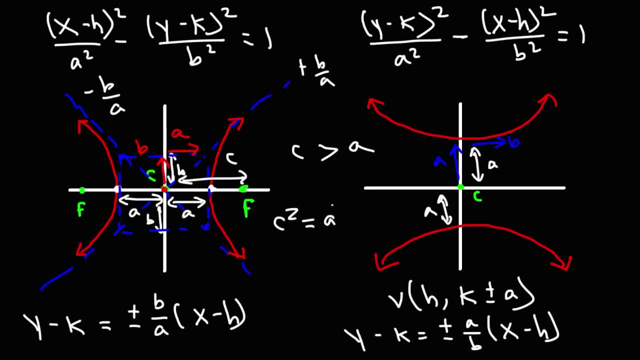 So c squared is going to be not a squared minus b squared, but a squared plus b squared. 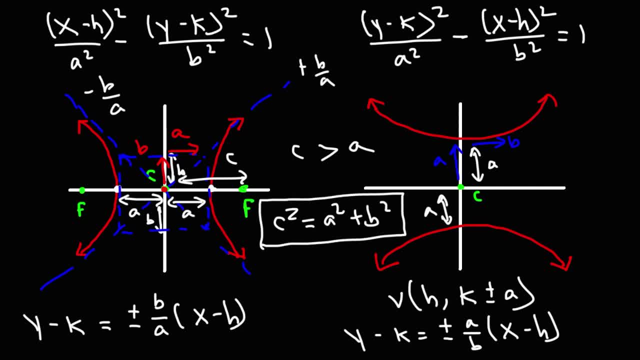 So for the hyperbola, this formula follows the Pythagorean theorem. 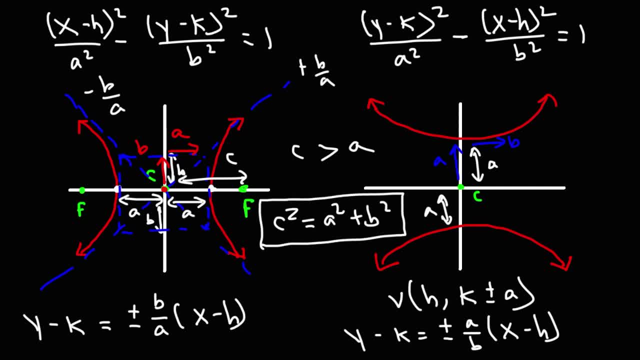 So for the hyperbola this is going to be. this formula follows the Pythagorean theorem, So that's how you could find C in order to find the coordinates of the foci. So that's basically it for the hyperbola. 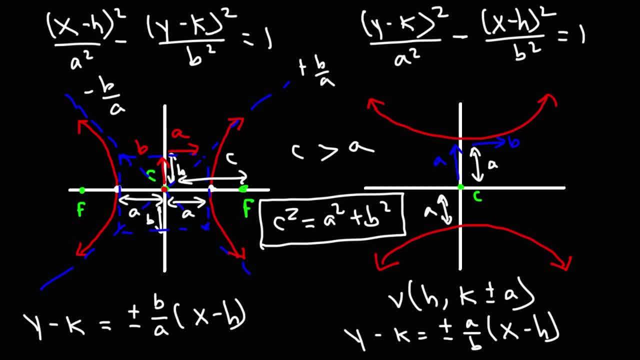 This is all you need to know in order to graph it and answer questions associated with it. And, once again, for those of you who want practice problems, check out the links in the description section below if you want to see some examples in terms of how to graph a hyperbola and other problems associated with hyperbolas. 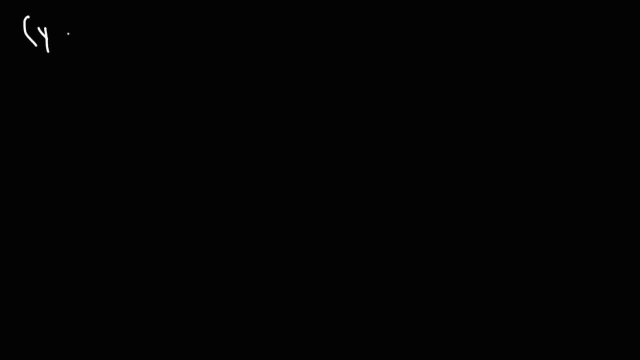 Now let's move on to parabolas. So let's start with this equation: Y minus K squared is equal to 4P times X minus H, And we can get two graphs associated with this equation. For the first one, the parabola can open towards the right You. 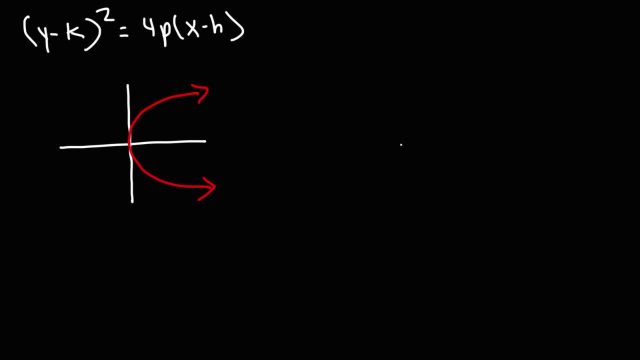 can think of the parabola as just one part of the hyperbola. It can also be open towards the left. the direction in which it opens depends on the p value. when p is positive, it's going to open towards the right. if p is negative, we're going to it's. 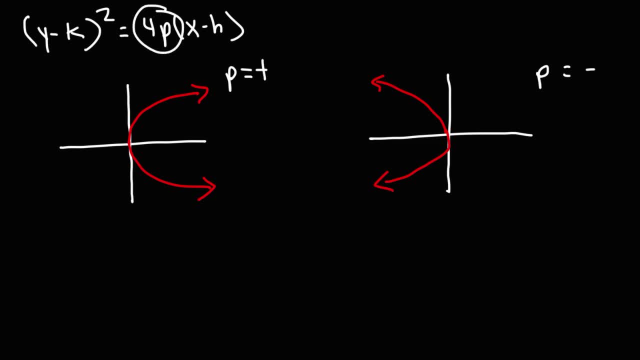 going to open towards the left. so it really depends on what you see here. if you were to see like, for example, negative 8 p would be negative. if you saw positive, 6 p is positive. now for the other equation, it's going to be x minus h. squared is equal to 4 p times y minus k. and for this, 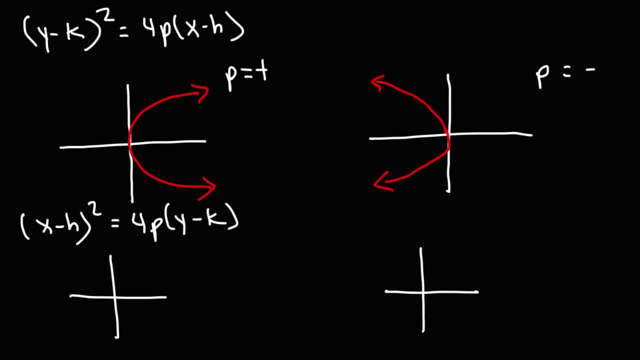 equation. it can either open upward or it can open downward. if it opens upward, p is positive. if it opens downward, p is negative. Oh, I think I showed you something. Now you might be wondering what can help me to remember these things. well, look at the formula. here we have x. x is not squared, but y is squared. so i think of this. 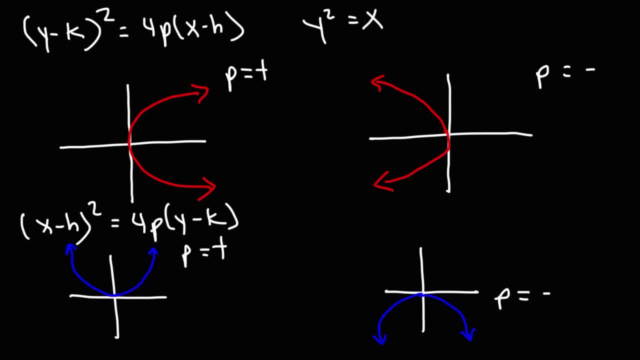 equation x is equal to y squared. for this formula, it's basically a parabola that opens left and right. for the other one, x is squared, y is not. so we get this equation: y is equal to x squared. you've seen this one I'm going to input either in the final part of the equation. 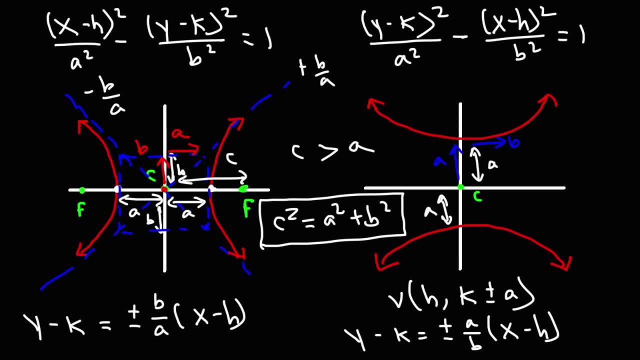 So that's how you can find c in order to find the coordinates of the foci. So that's basically it for the hyperbola. 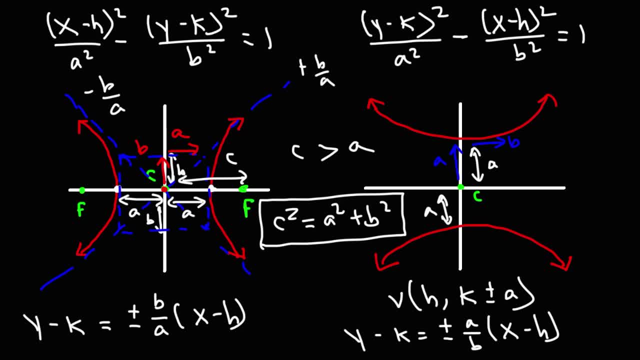 This is all you need to know in order to graph it and answer questions associated with it. And once again, for those of you who want practice problems, check out the links in the description section below if you want to see some examples in terms of how to graph a hyperbola 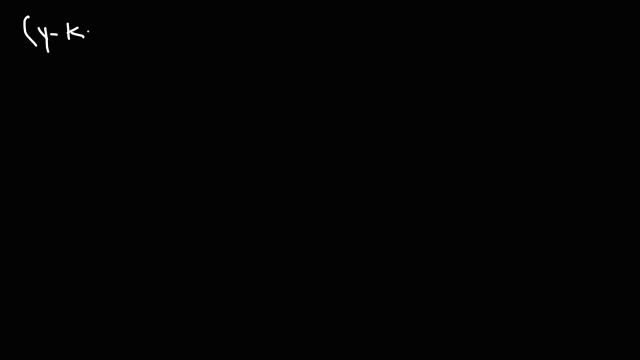 Now, let's move on to parabolas. So let's start with this equation. 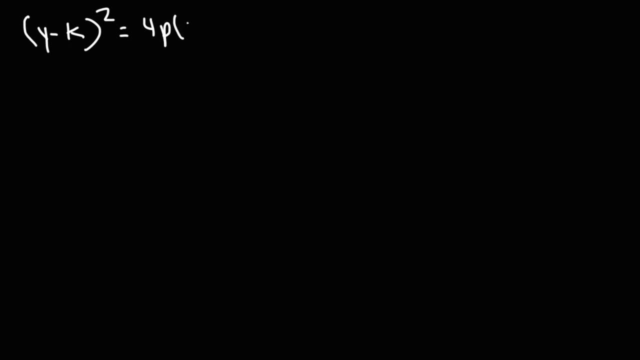 y minus c. y minus c. y minus c. y minus k squared is equal to 4p times x minus h. 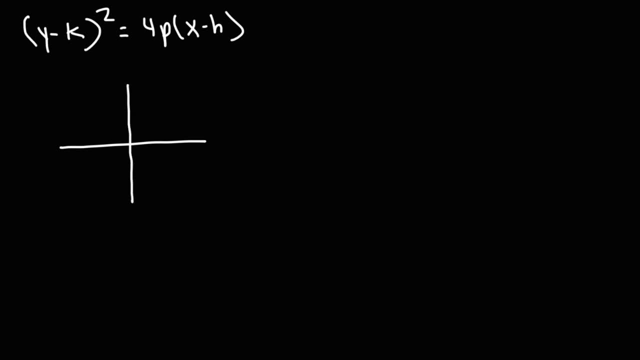 And we can get two graphs associated with this equation. For the first one, the parabola can open towards the right. You can think of the parabola as just one part of the hyperbola. 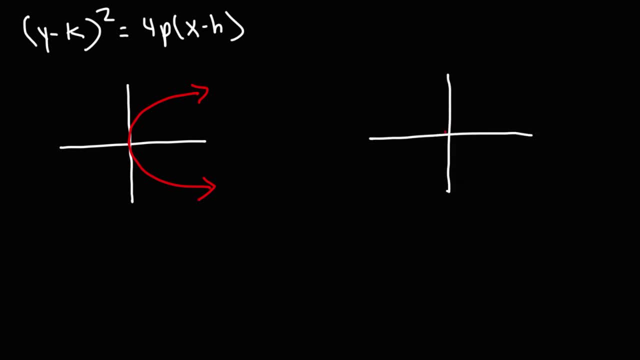 It can also open towards the left. The direction in which it opens depends on the p-value. When p is equal to 1, when p is positive, it's going to open towards the right. 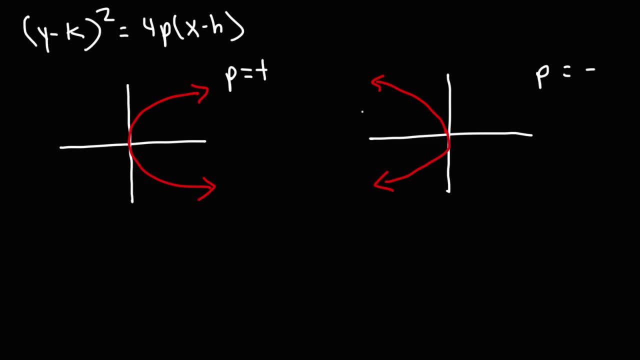 If p is negative, it's going to open towards the left. So it really depends on what you see here. 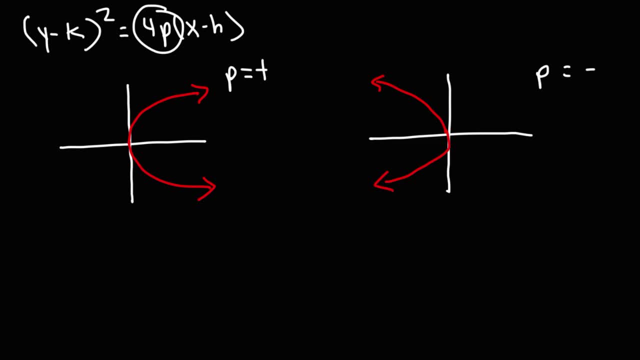 If you were to see, like, for example, negative 8, p would be negative. If you saw positive 6, p is positive. 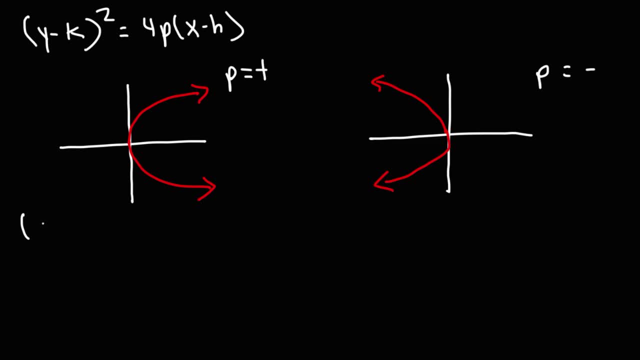 Now, for the other equation, it's going to be x minus h squared is equal to 4p times y minus k. 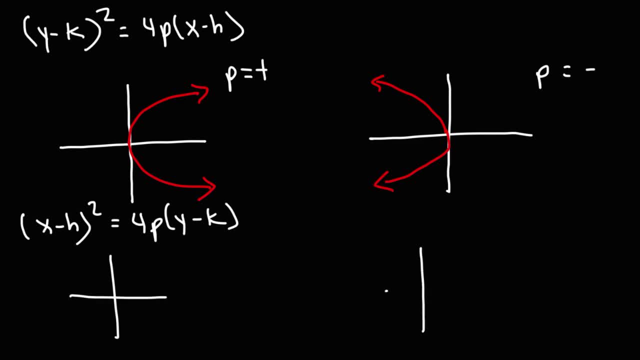 And for this equation, it can either open upward or it can open downward. 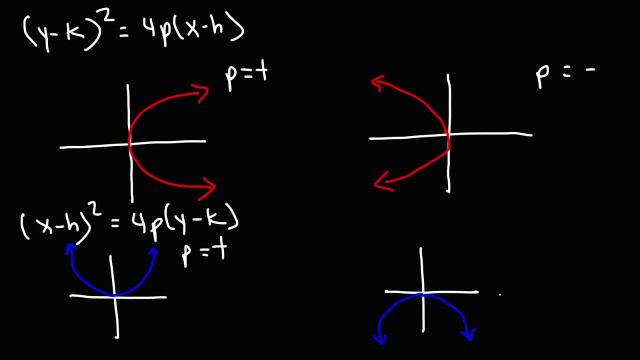 If it opens upward, p is positive. If it opens downward, p is negative. 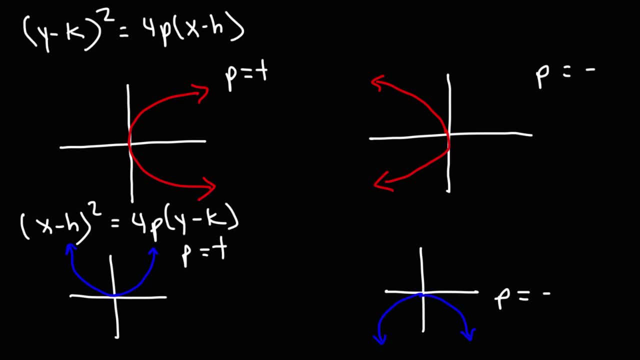 Now, you might be wondering, what can help me to remember these things? Well, look at the formula. Here we have x. 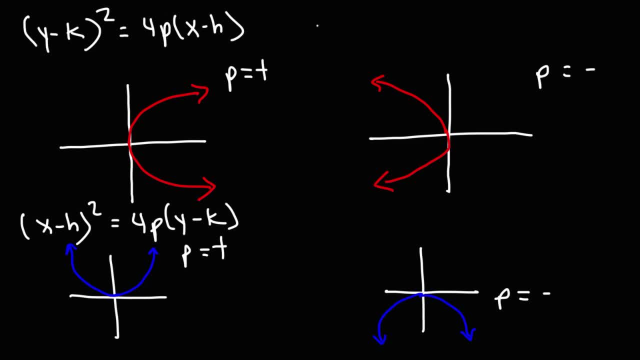 x is not squared, but y is squared. So I think of this equation. x is equal to y squared. 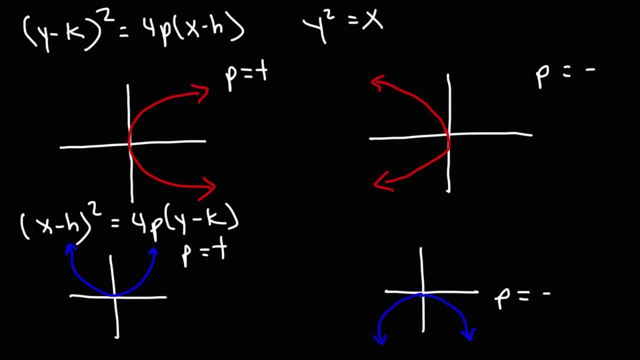 For this formula, it's basically a parabola that opens left and right. 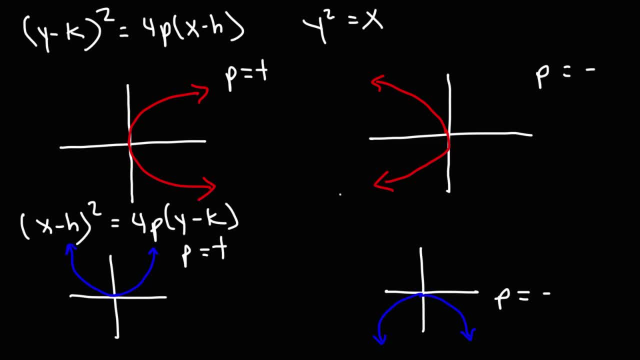 For the other one, x is squared, y is not. So we get this equation, y is equal to x squared. 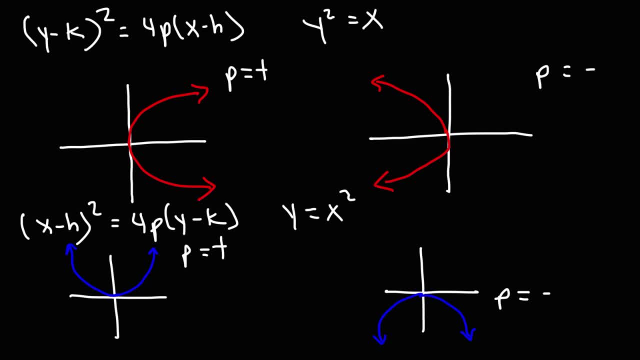 You've seen this one, either in the form of a quadratic equation or a parabola. 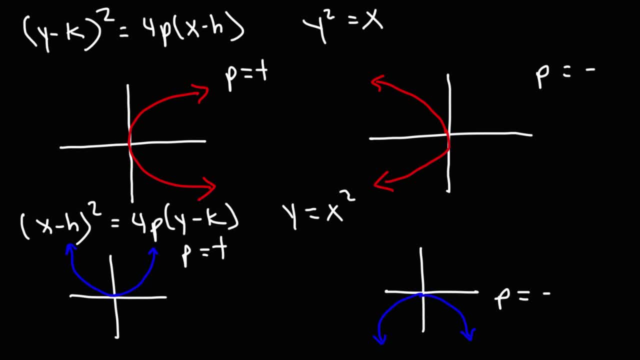 If we have y equals positive x squared, we know we have a parabola that opens upward. If it's y equals negative x squared, it opens downward. So that can help you to remember the direction. 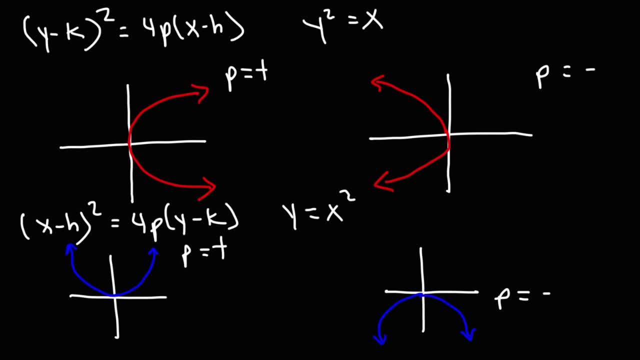 So when we have x equals y squared, it opens either to the left or to the right. But if you have y equals x squared, it opens up or down. 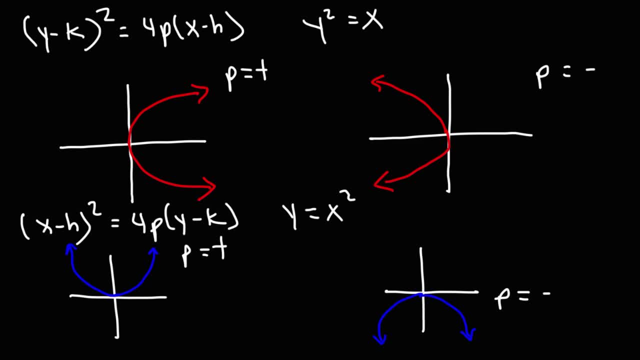 Now, we need to talk about how to find the equation of the directrix and the focus. 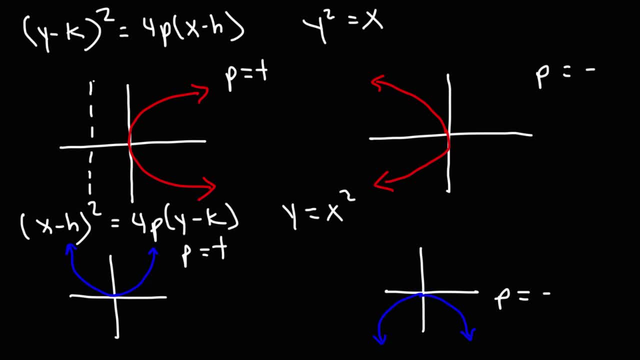 So, the directrix is always away from wherever the parabola opens up, and the parabola, it always opens towards the focus. 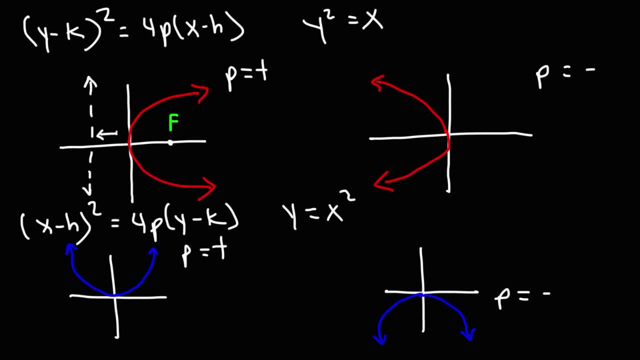 The directrix opens up the parabola. The parabola opens up towards the focus. The directrix is p units away from the vertex, and the focus is also p units away from the vertex. 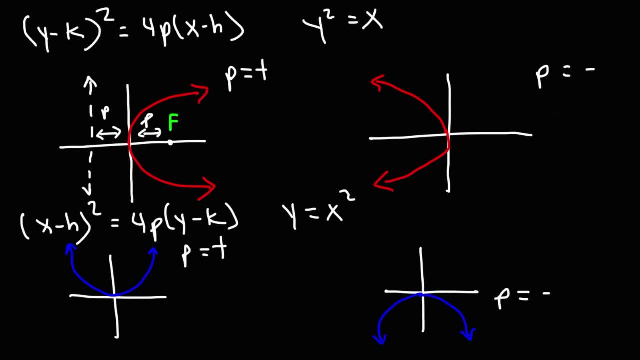 So one of the first things you need to do is find the center, which is h comma k, and then calculate the value of p. 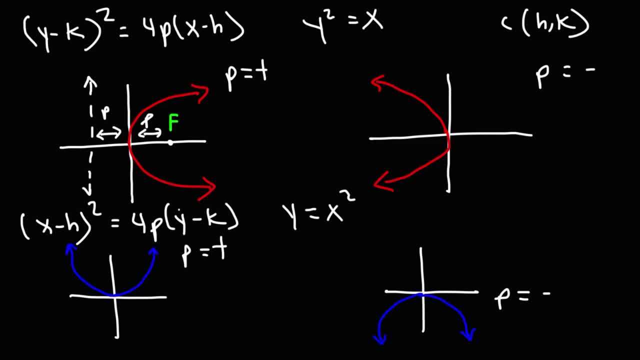 Because once you have p, you can find the equation of the directrix and the coordinates of the focus. 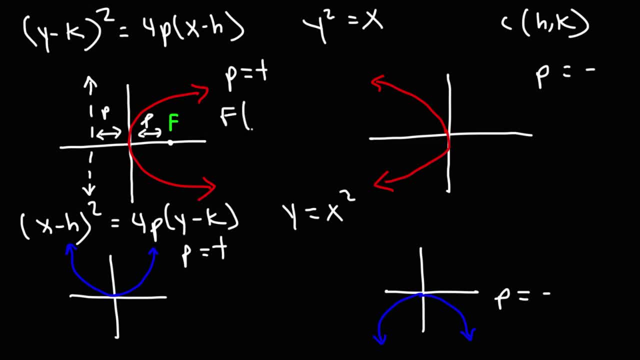 So for the graph at the top left, the coordinates of the focus is going to be the center, h, and then since we traveled p units to the right, it's going to be h plus p, and then comma k. 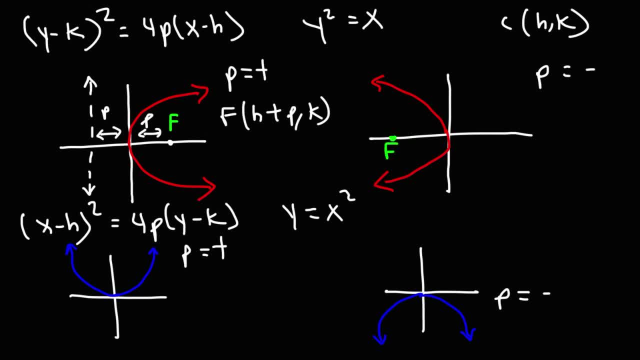 For the next graph on the right, the coordinates of the focus is going to be h minus p, because we went p units to the left from h, and then comma k. 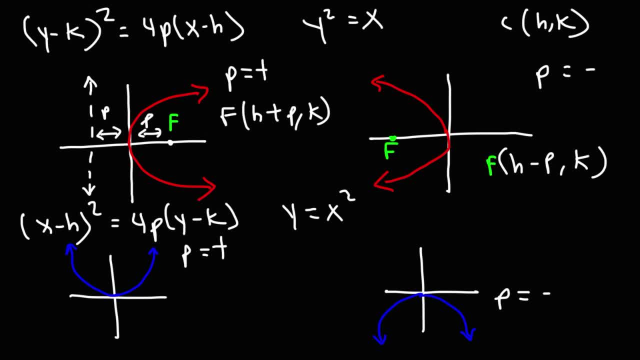 So that's the... That's the coordinates of the focus for the graph on the right. 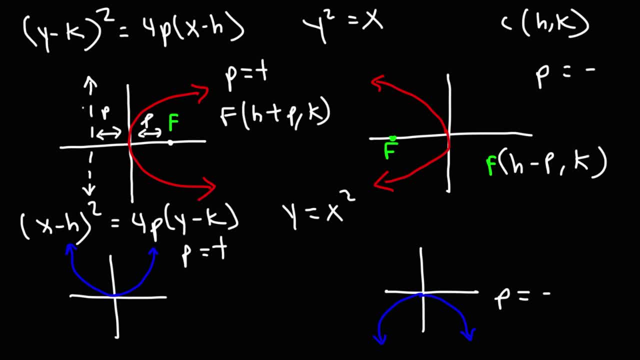 Now for the equation of the directrix, since we have a vertical line, it's going to be x equals. 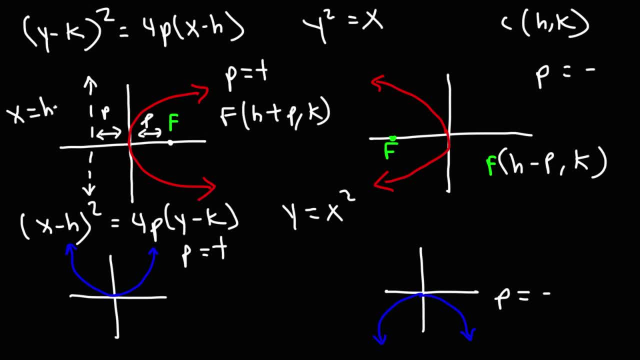 So it's x equals h minus p. 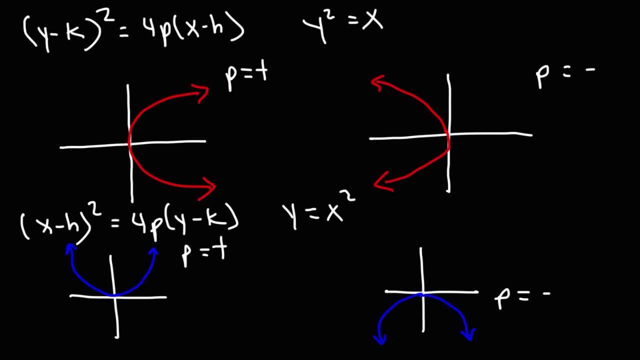 There'szin a camera for that, and this is at the end of the equation, form of a quadratic equation or a parabola. If we have y equals positive x squared, we know we have a parabola that opens upward. If it's y equals negative x squared, it opens downward, So that 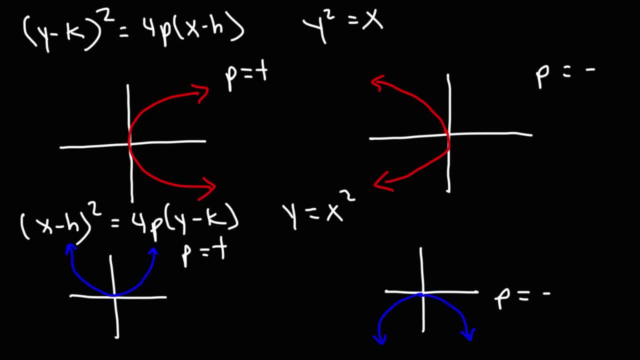 can help you to remember the direction. So when you have x equals y squared, it opens either to the left or to the right, But if you have y equals x squared, it opens up or down. Now we need to talk about how to find the equation of the directrix and the focus. So the directrix is always. 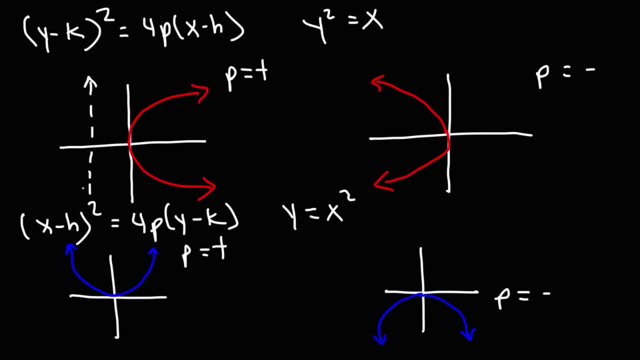 away from wherever the parabola opens up- And the parabola, it always opens towards the focus. The directrix is p units away from the vertex And the focus is also p units away from the vertex. So one of the first things you need to do is find the center, which is 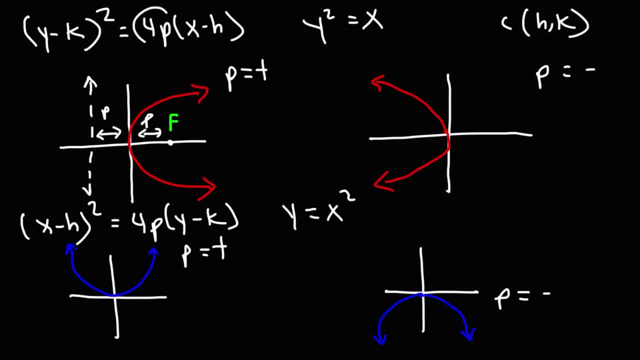 h, squared comma k, and then calculate the value of p, because once you have p you could find the equation of the directrix and the coordinates of the focus. So for the graph at the top left, the coordinates of the focus is going to be the center h and then, since we travel p units to the right, it's going to 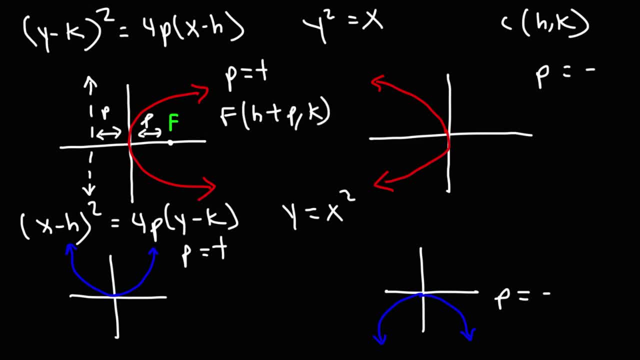 be h plus p and then comma k. For the next graph on the right, the coordinates of the focus is going to be h minus p, because we went p units to the left from h and then comma k. So that's the coordinates of the focus for the graph on the right. Now for the equation of the directrix. 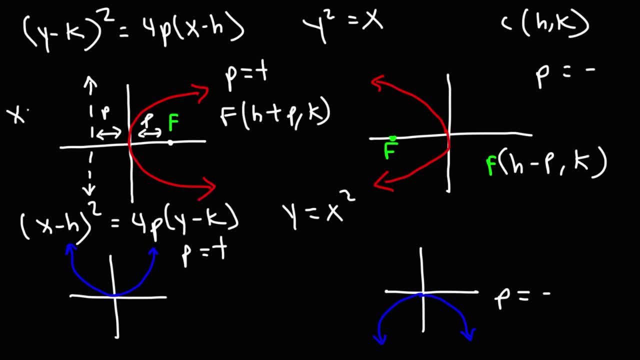 since we have a vertical line, it's going to be x equals. So it's x equals h minus p. Here we have the other equation of the directrix and it's going to be: x is equal to h plus p, since we traveled p units to the right from the center. 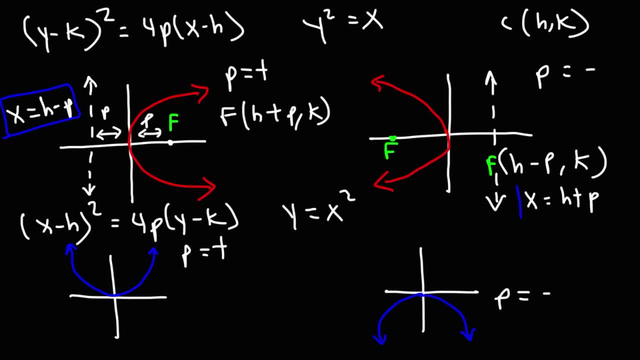 So these are the equations of the directrix for the first two graphs. Now let's move on to the vertical line. So it's going to be x equals h minus p- the bottom ones. So the equation of the directrix is going to be different. The directrix is now: